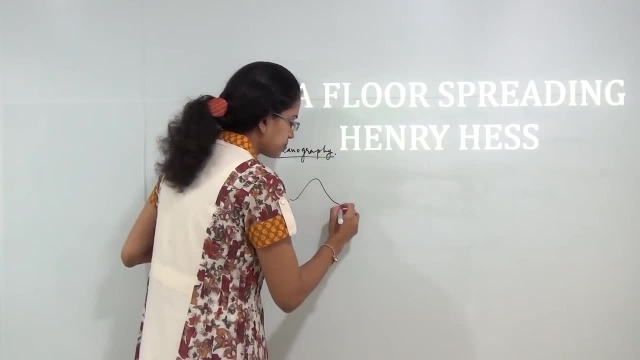 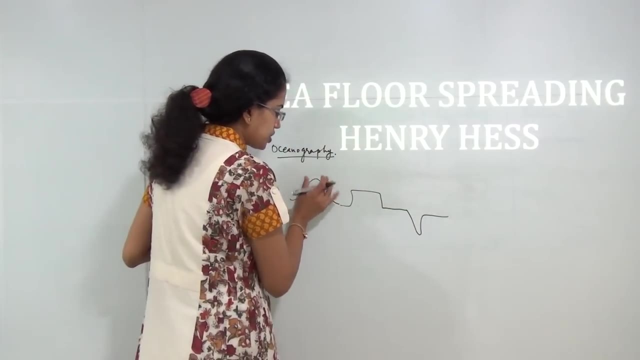 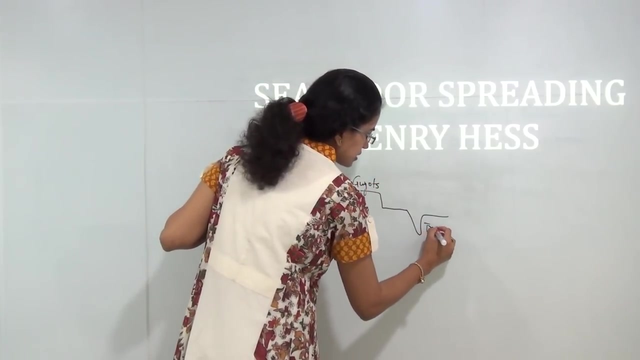 our land and you have kind of mountains, you have flat topped hills and you have deep trenches. So these are known as ocean ridges, these are known as guillots and these are the trenches that are found mainly in the ocean reef. So ocean relief, when we talk about, we have these. 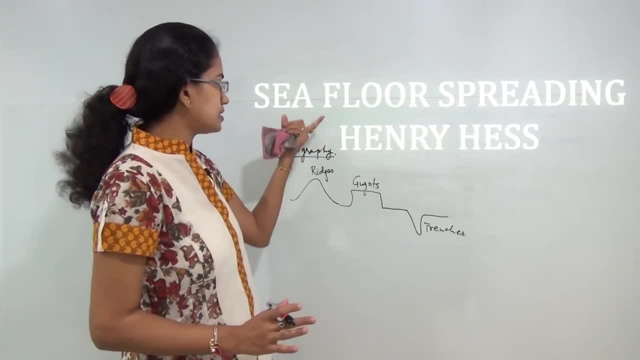 three main concepts. So we have the ocean relief, we have the seafloor spreading, we have the seafloor drift and we have the seafloor drift. So these are the main features that we will try to incorporate in this class. Along with that, we will try to understand 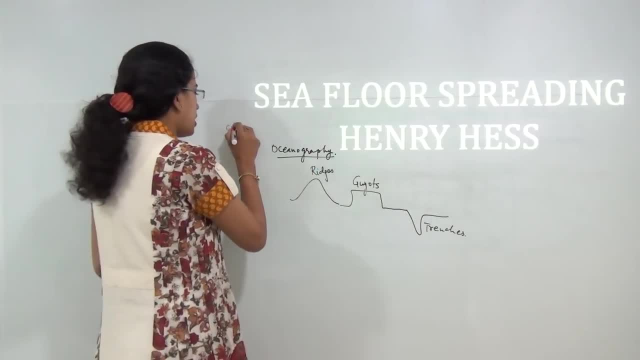 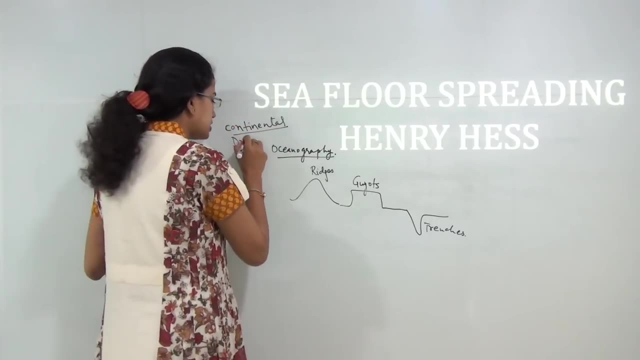 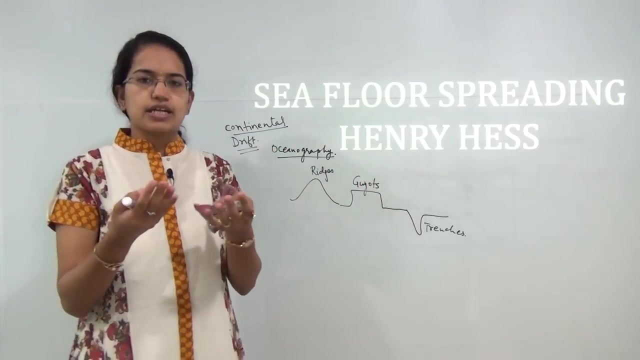 the previously discussed continental drift theory. So now, why was seafloor spreading concept introduced and what was the reason that continental drift theory was criticized? Wegener gave the continental drift theory where he said the earth was a kind of one mass and it slowly drifted away. 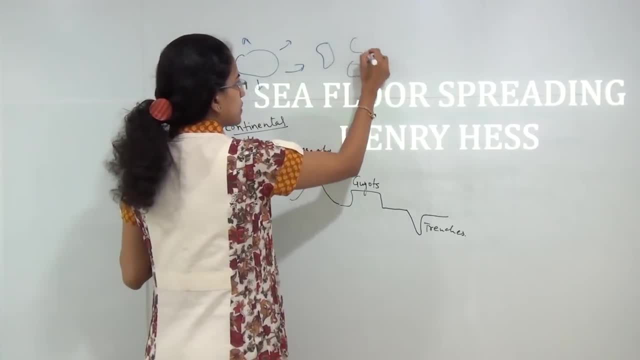 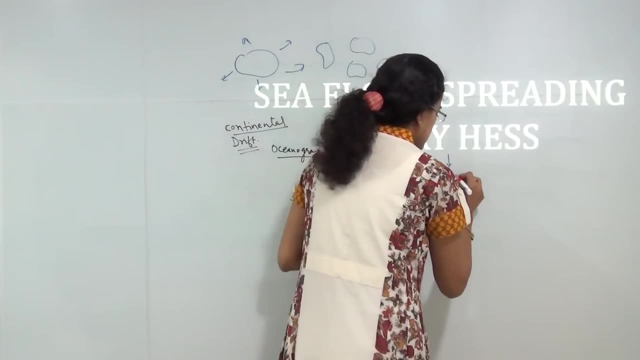 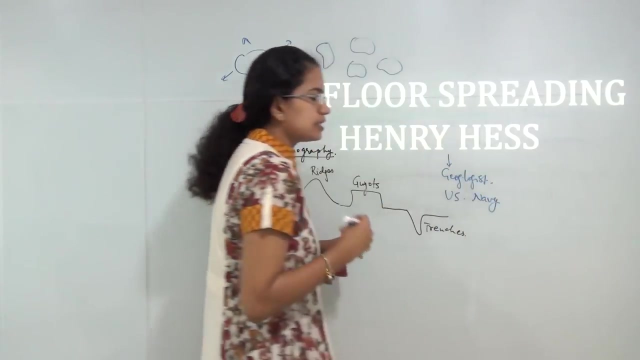 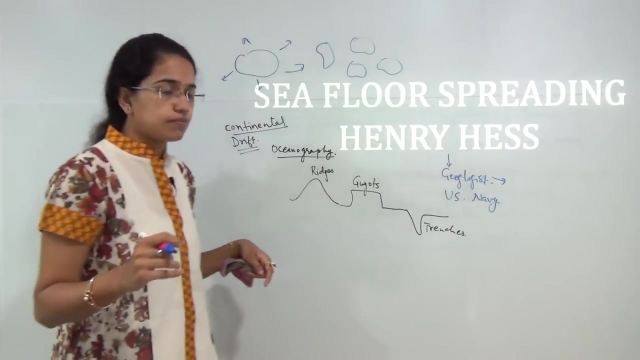 And there were continents formed individually. So that was what Wegener explained. But Henry Hess, who was basically a geologist and also a US Navy Admiral, did many researches of the ocean bottom during World War II to understand the locations of the enemy submarines. So 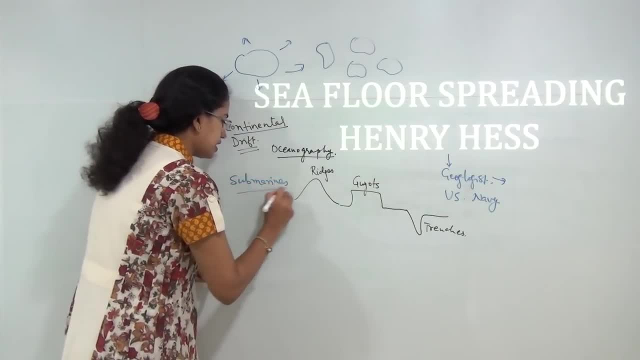 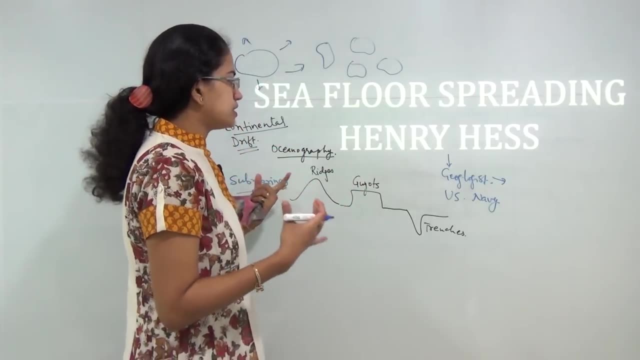 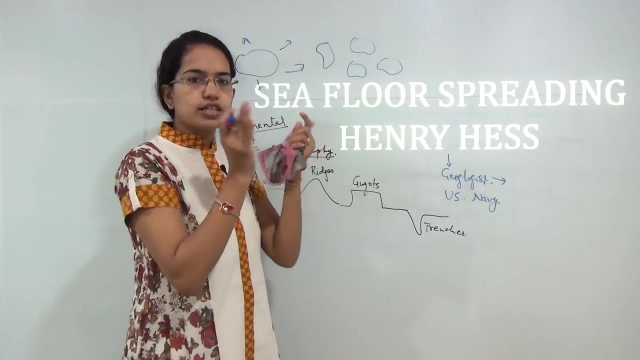 to understand those locations of the submarines. he did extensive researches, He did extensive study of the ocean bottom floor and while studying the ocean bottom floor he came up with certain phenomena and he said that it is not really that the continent is dividing or there is one land mass that is breaking down. rather it is the seafloor. 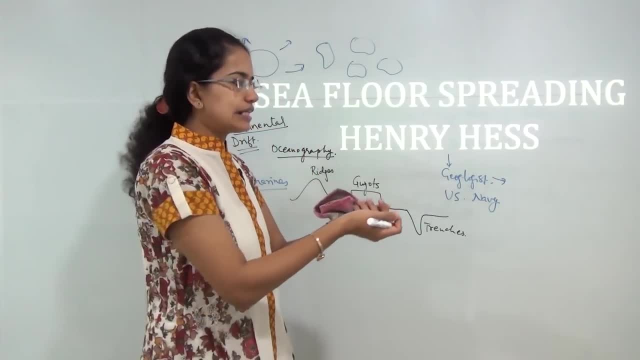 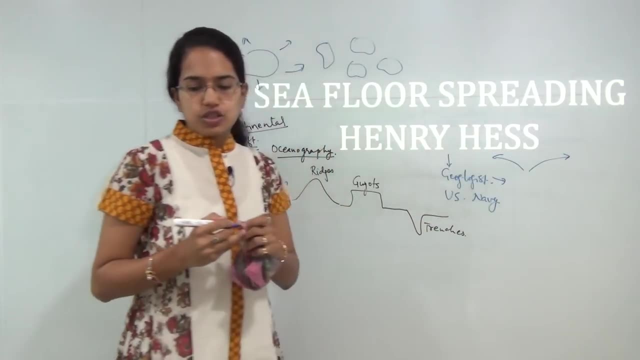 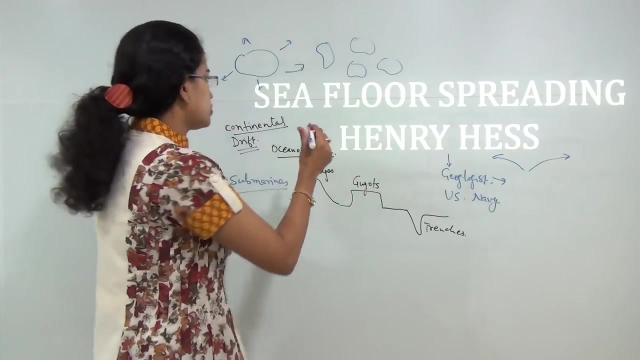 or the floor of the ocean that is slowly and gradually expanding and because of that expansion continents are drifting away. So, in very simple terms, He said there is new seafloor that is being added to the lithosphere. So I can say it's. 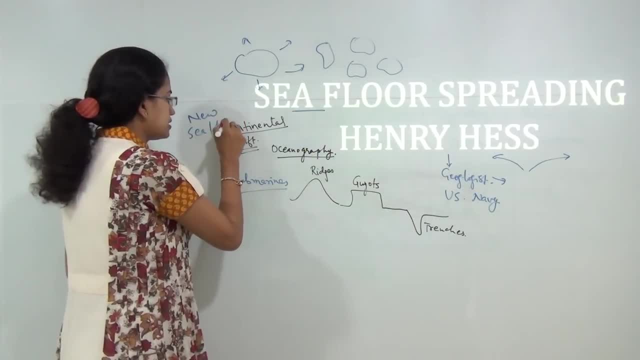 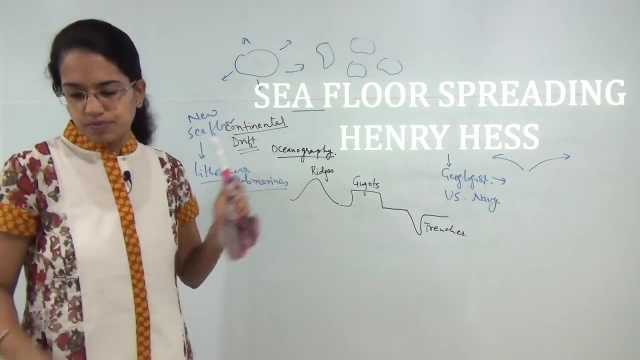 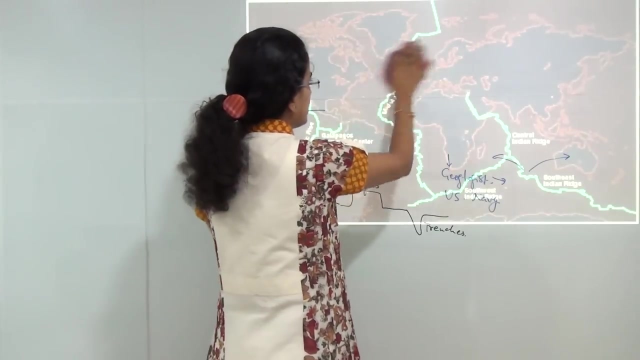 new seafloor, and this new seafloor is being added to lithosphere. So that was the basic idea, what Henry Hess proposed. Now, coming on to this world map, you have the lines with blue color that indicate the major ocean ridges. So, as you can see, the various plates and the lines with blue color indicate the major ocean. 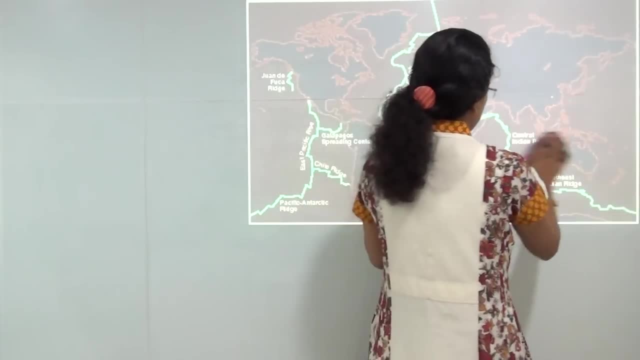 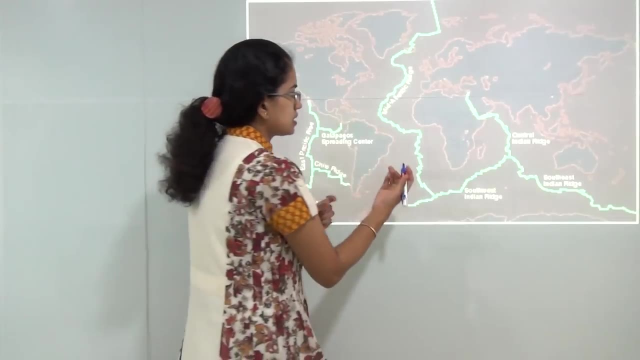 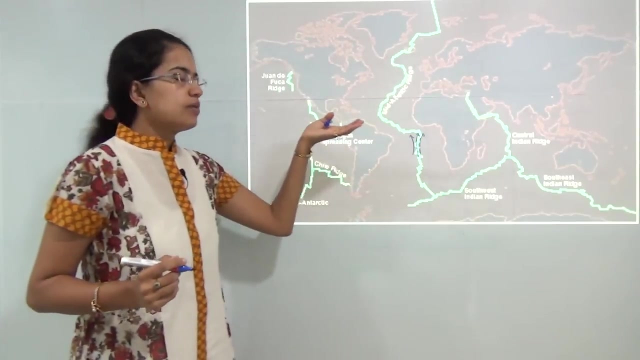 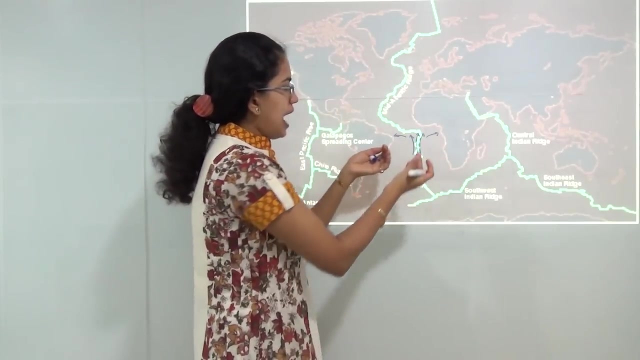 ridges. What has propounded was: at the region of this ridge there is volcanic material or molten magma that drifts up. Because of that, you have the two plates that move apart and since, because of this, there is pushing of the surface A great deal. 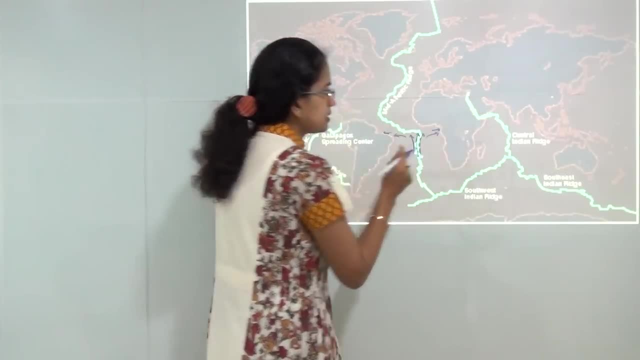 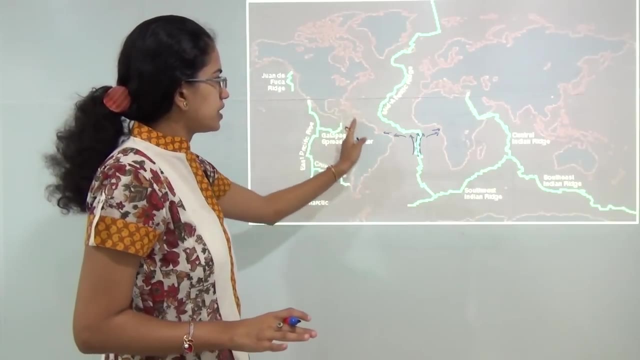 So the pits move freely So that you can see the two plates. So now you can imagine a very big TEDx conference, both the continents that are being drifted apart. So what he propounded was, if there is a region with trench nearby, okay, this region would. 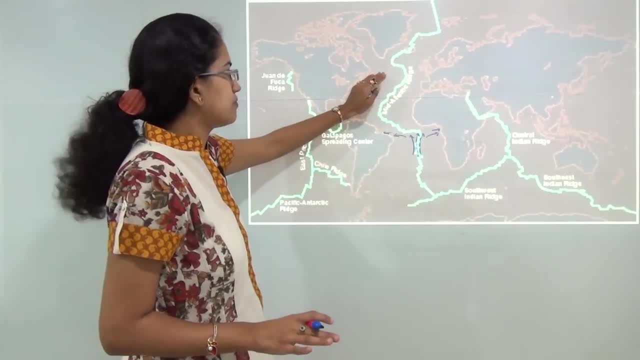 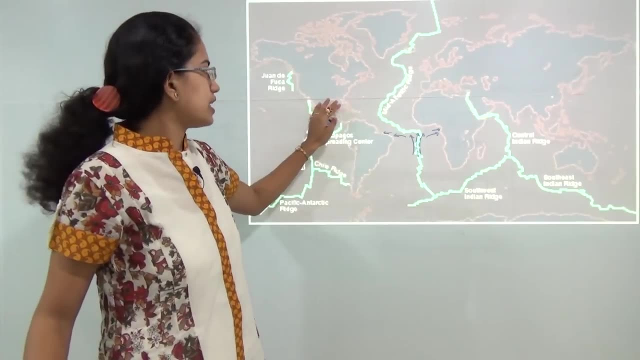 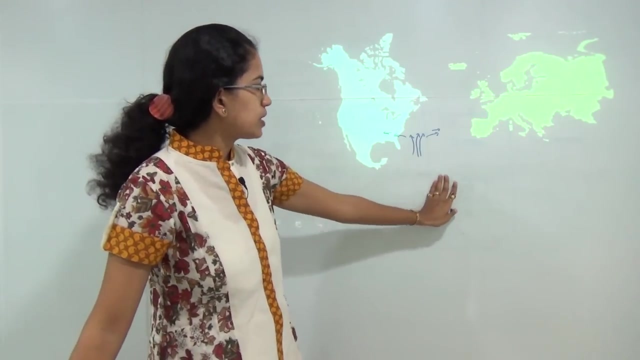 slowly and gradually be pushed apart. but if there is no deep trenches, there would be kind of slow movement as compared to the other case. so, as you can see, here you have Eurasia and North America. what he propounded was: because of the mid-Atlantic ridge, you have molten. 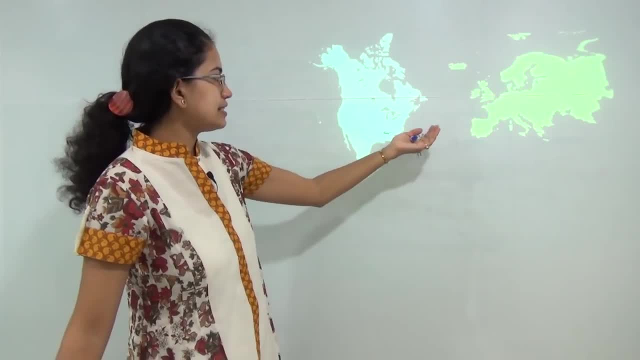 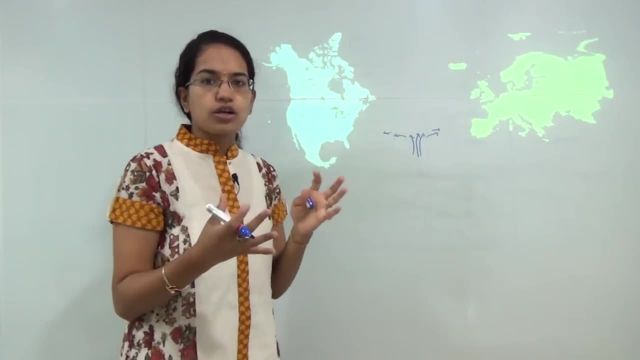 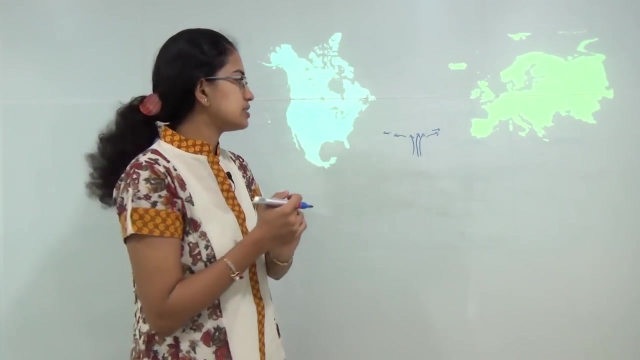 magma that's coming through here and the sea floor is spreading. as a result, you can see the two continents drifting apart. So he said the idea was not what Wigner proposed under the continental drift theory, where he said one landmass breaks up into different landmasses, but rather it's the sea floor. 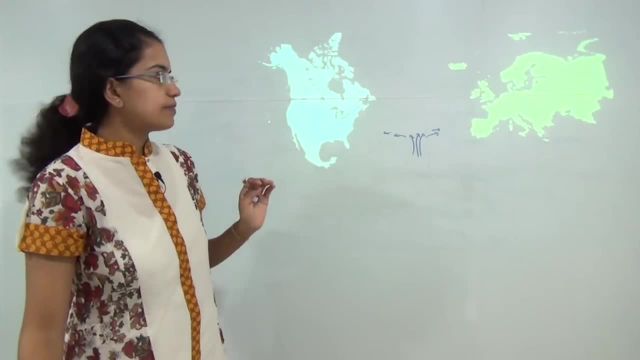 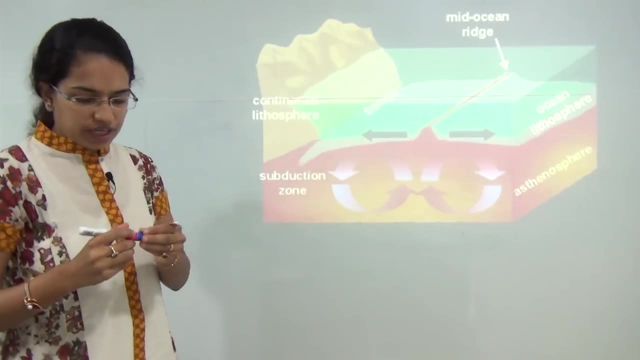 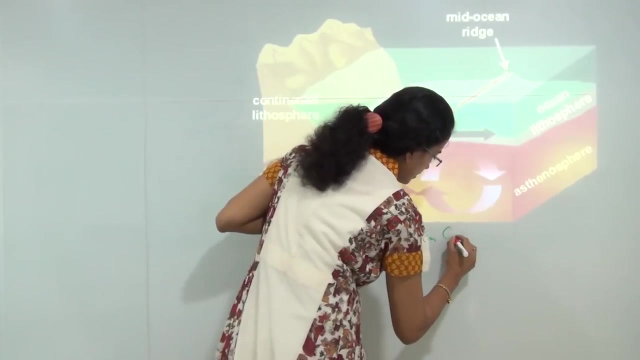 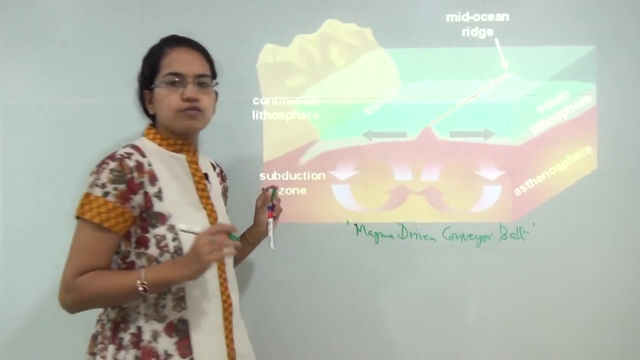 that is kind of pushing apart. Okay, It's pushing the continents apart. So, to understand this, he tried to explain the concept of magma driven conveyor belts. So he talked about magma driven conveyor belts. Now, this is the main essence of the whole idea of sea floor is spreading and you must. 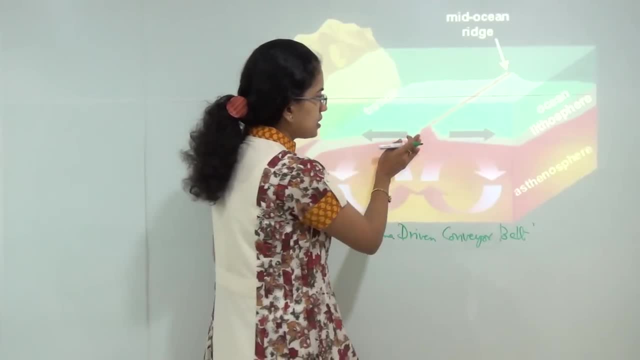 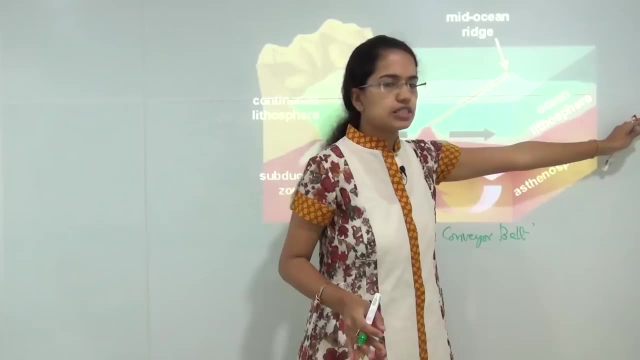 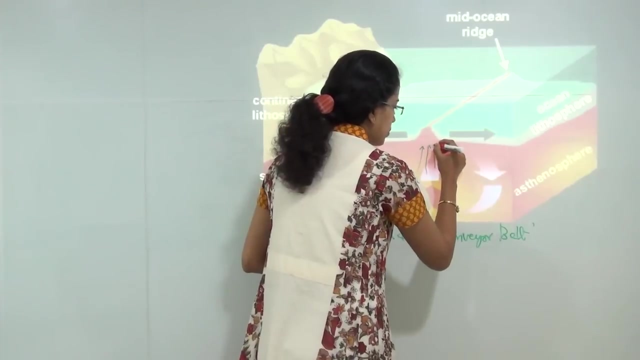 be very, very clear with it. So let's start. This region is the ridge. Let's say: this is the mid-Atlantic ridge. you have North America on one side and you have Eurasia and Africa on other side. what is happening here is you have molten magma that flows up. 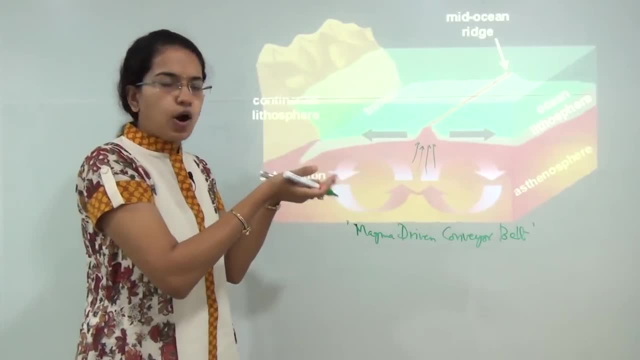 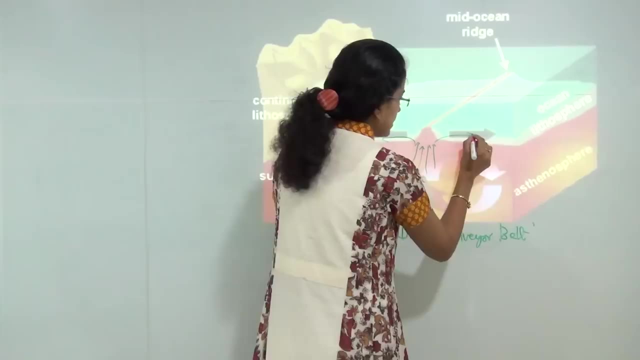 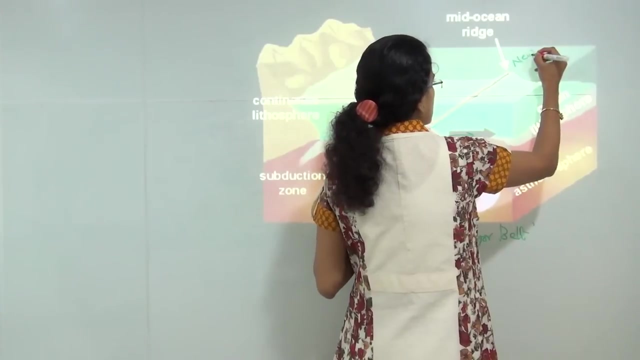 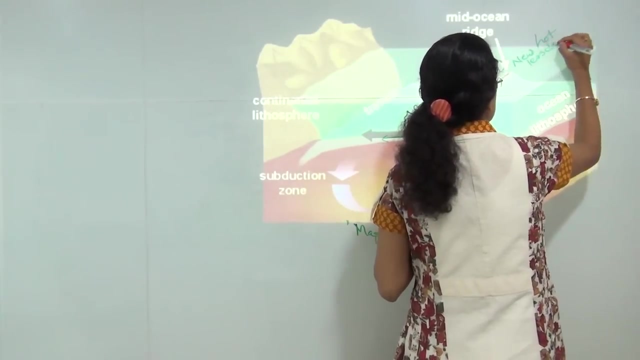 when the molten heat and hot magma goes up it tries to spread out on either side. So when it is spreads, the region towards the center has new rocks and new rocks and new rocks On new formations. it is hot and it is less dense. 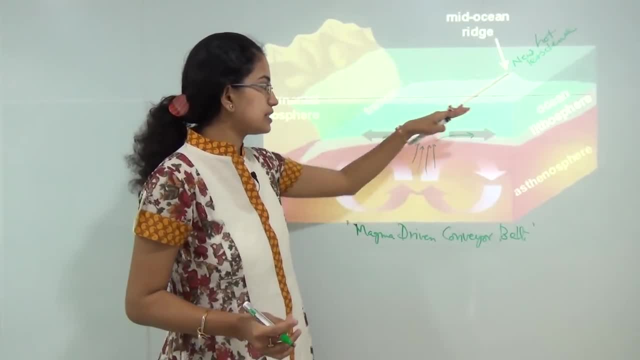 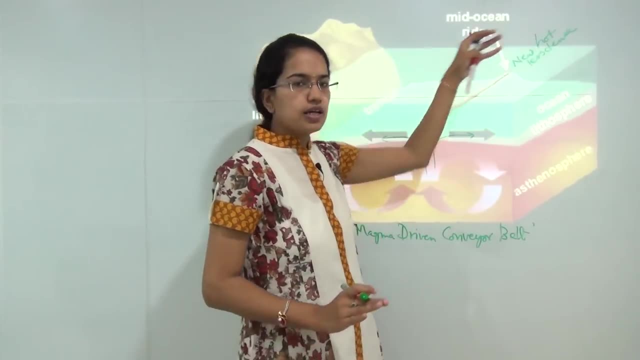 So these three things are to be noted very precisely towards the center, where the hot magma is rising, since it's hot, this region would be hot. This is newly formed region and it is less denser than the surrounding region, as in when the plates move apart. 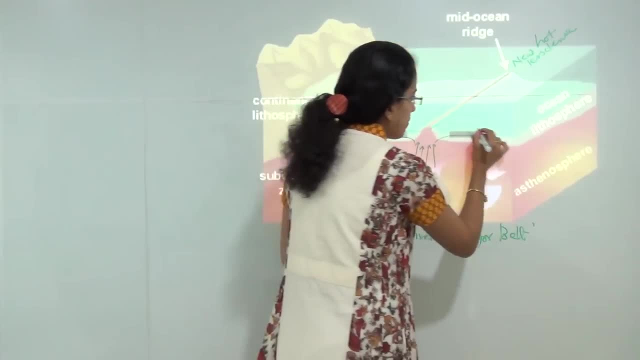 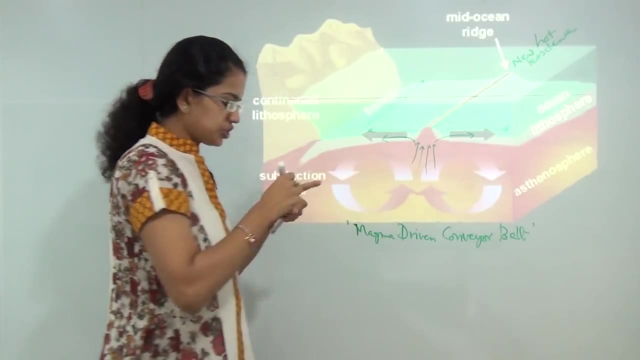 This region is hot. This region is newly formed region and it is less denser than the surrounding region As in when the plates move apart. This region is hot. On the c Flores spreads the region which is away from the mid-Atlantic ridge. the region 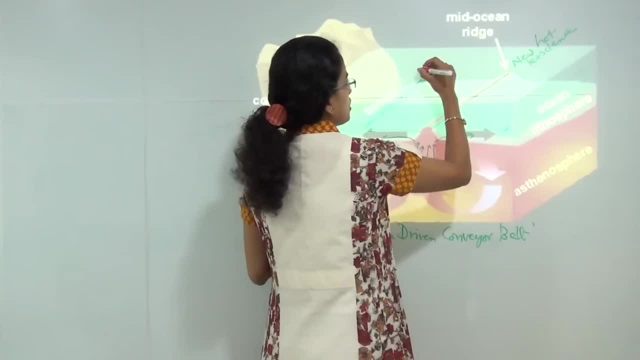 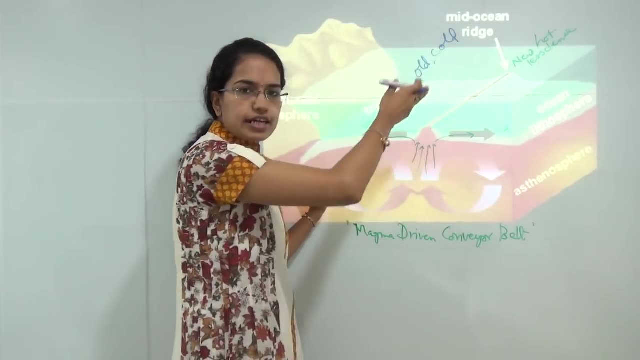 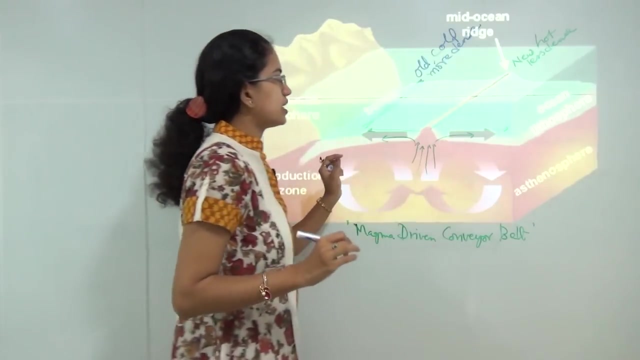 that is far away from mid-Atlantic ridge would be having older rocks, it would be much cold as compared to the center of the mid-Atlantic ridge and it would also be more dense. So these two things to be very clear about the mid-Atlantic region or mid-Atlantic ridge. 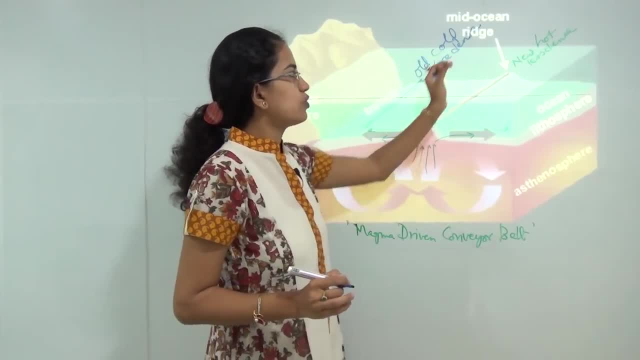 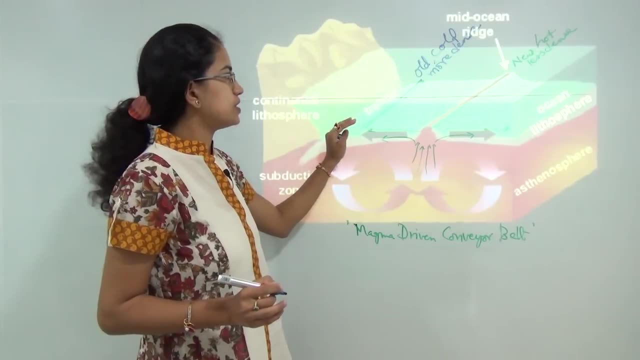 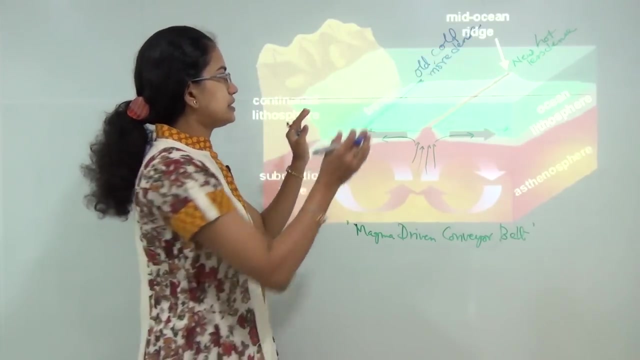 ridge where the magma is erupting up would be new, it would be hot and less dense and the region away from the mid-atlantic ridge, as I said previously, would be old, would have colder region and would be more dense. now, since that is cold and more dense, it would try to subside down, so there would be subduction. 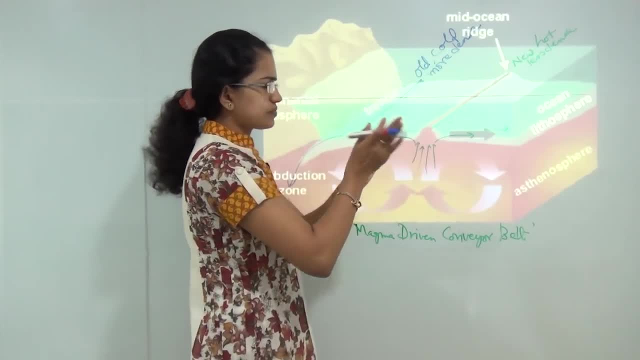 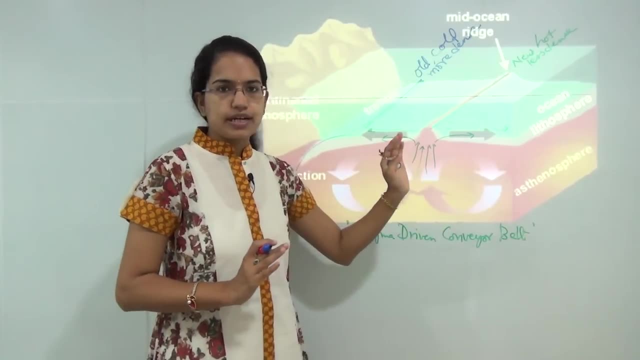 that would occur here. so what is happening here is it's a kind of volcano that if it is erupting under the ocean, it would be towards the mid-atlantic ridge, but if it is towards the coast it would come out in the form of volcano. so when it erupts, the hot magma moves up. the center region where the hot magma is coming up would be hot and it would be less dense, but as it goes away from the core of the magma rising, this region would be colder. it would be more dense, since it is cold and more dense. 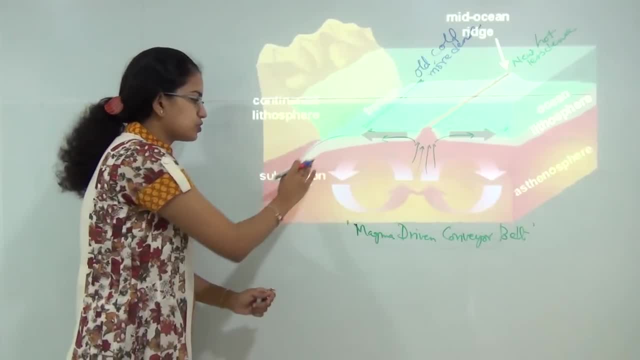 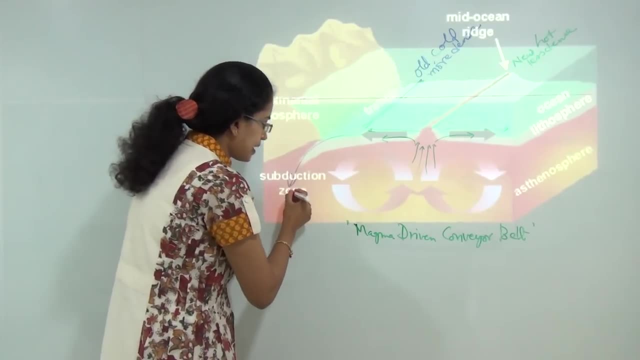 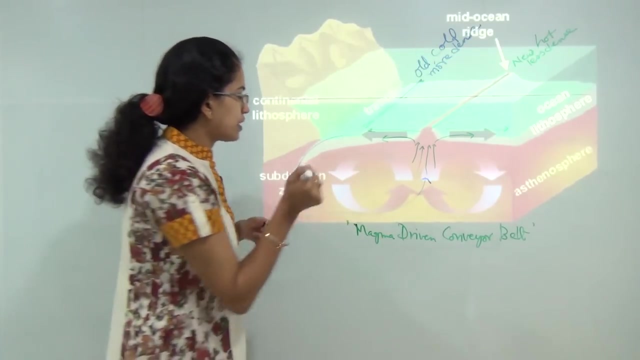 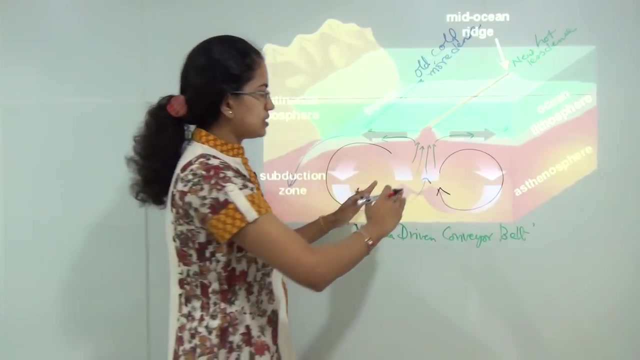 it would tend to subside, so this region would be the zone of subduction. so what would happen here is the magma would go down and this magma would again form the kind of conveyor belt. so what we call here is the magma driven conveyor belt, as you can see. so what is happening is magma is rising here, going towards the 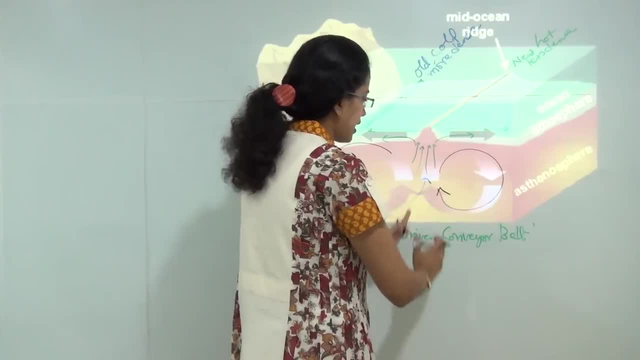 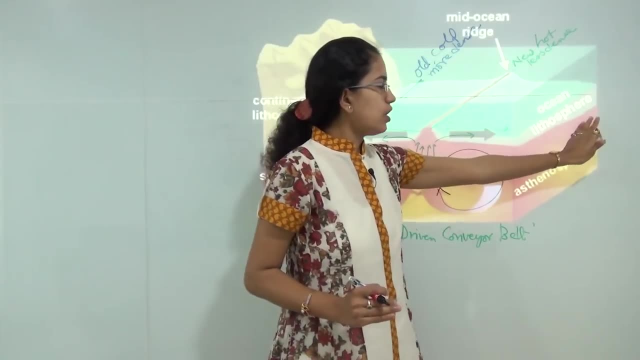 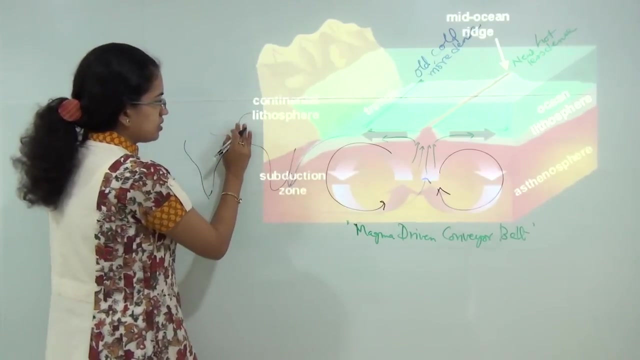 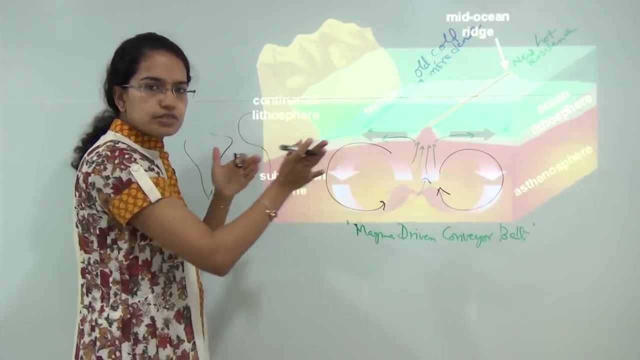 subduction zone, so getting suppressed and then again leading to the formation of magma here. So this is how it goes on and on. So if we talk about the South American coast and the African coast, the coast towards Africa does not have many trenches. As a result, there would be higher pressure of spreading in this. 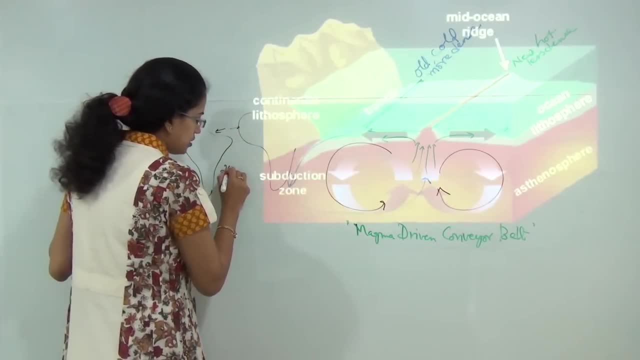 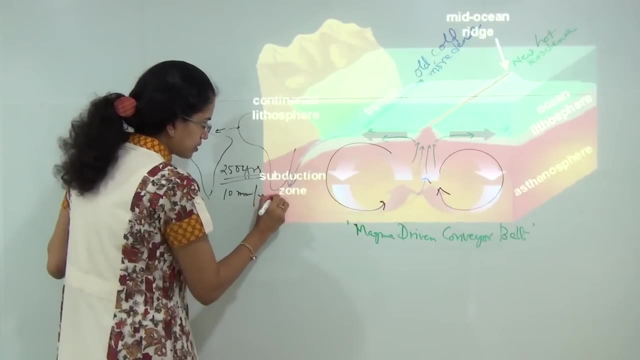 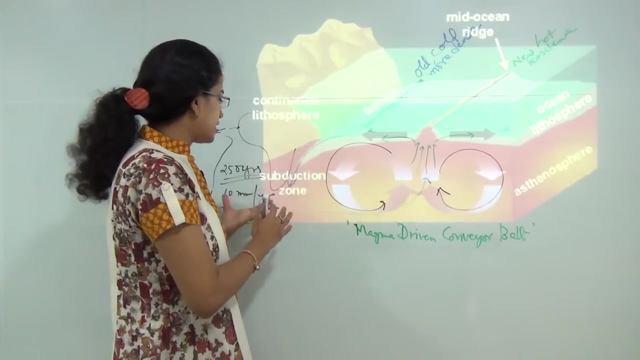 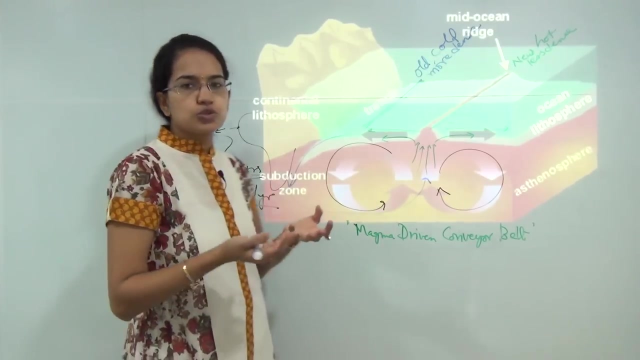 region. So it is said, around in last 250 years there has been a drift of 10 mm per year approximately and these two continents have drifted apart based on this rate. So he said that this drifting is not due to what Wegner proposed into the continental drift theory, but it is due to. 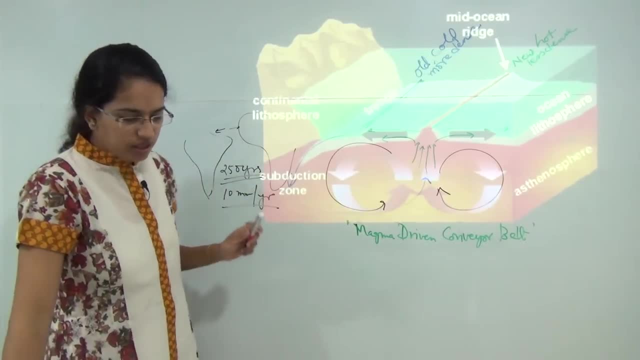 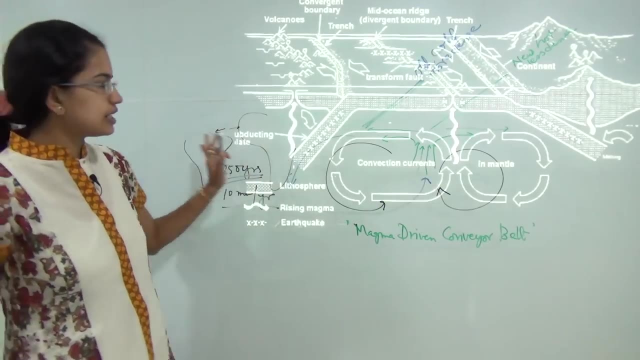 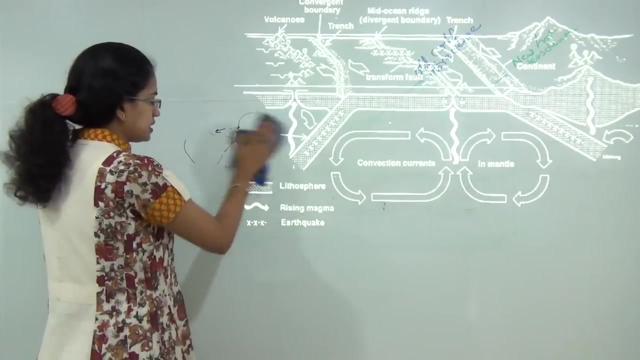 the spreading of the ocean bottom. So this is how the Hohmann's law is taught. This is how the Hohmann's law is taught. whole mechanism of seafloor spreading works now, as you can see in another diagram. here you have the convention currents that are going in the mantle. so these convention currents, 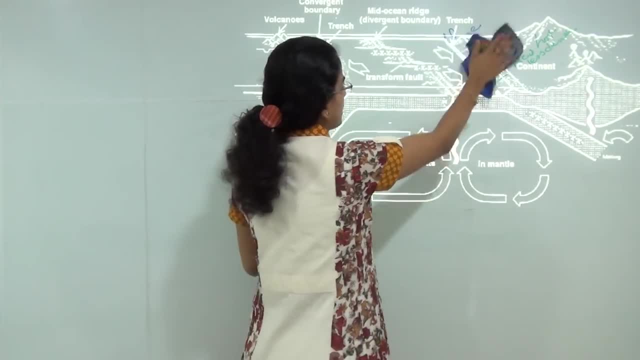 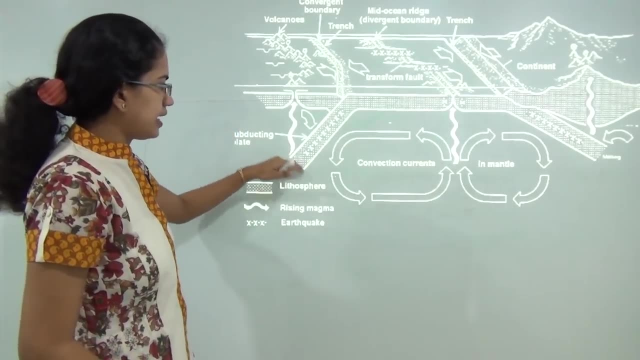 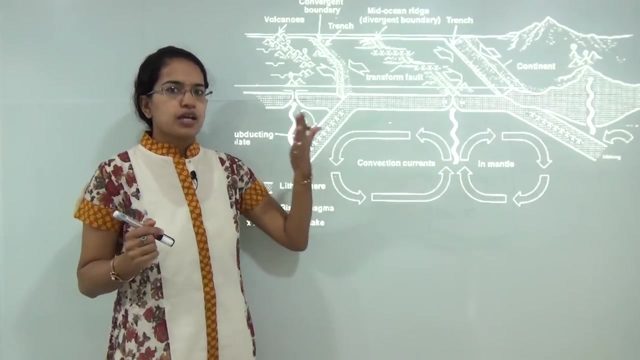 what they do is they affect the mantle and the core and finally you have the hot magma rising that takes place here. you can see the subduction zone here and again the rising magma, as i explained previously. so, according to uh henry hess, atlantic ocean is spreading. 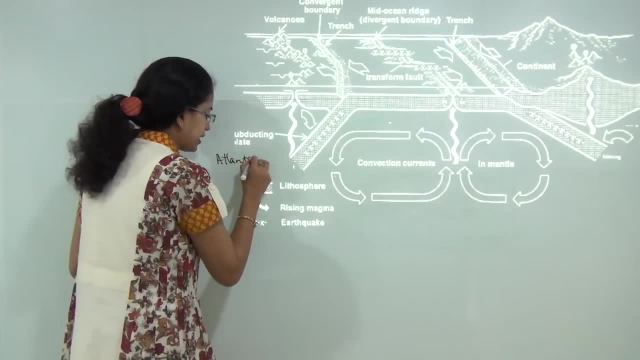 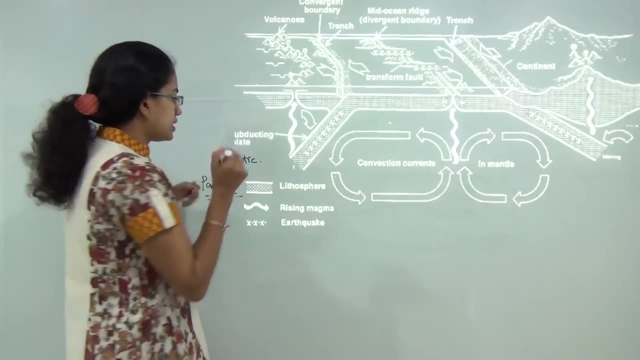 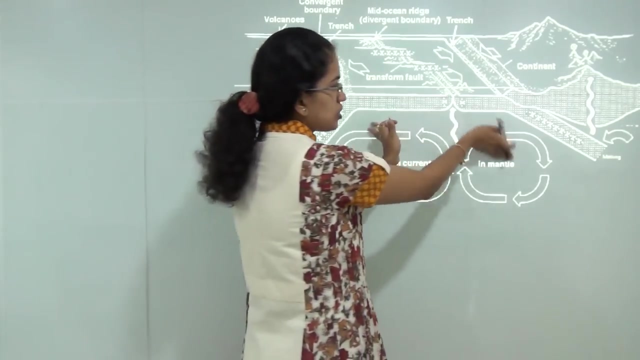 so atlantic, he suggested, was spreading, but on the other hand pacific ocean is shrinking. since there are no trenches in the atlantic ocean, it's not subsiding. the whatever magma is rising is not going in. so it's kind of spreading or helping the contact with the 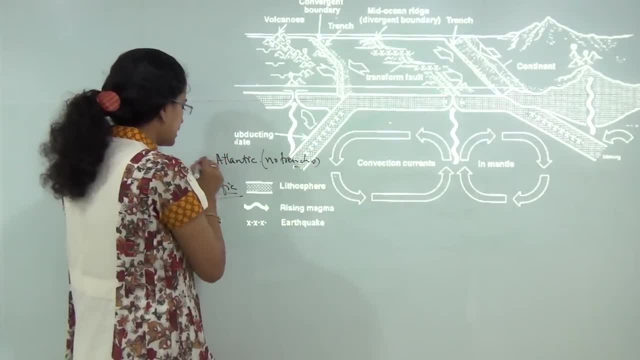 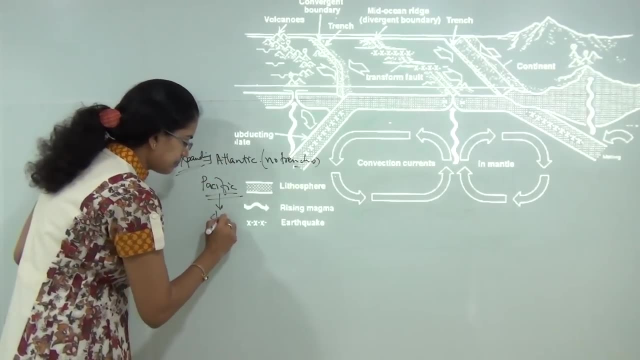 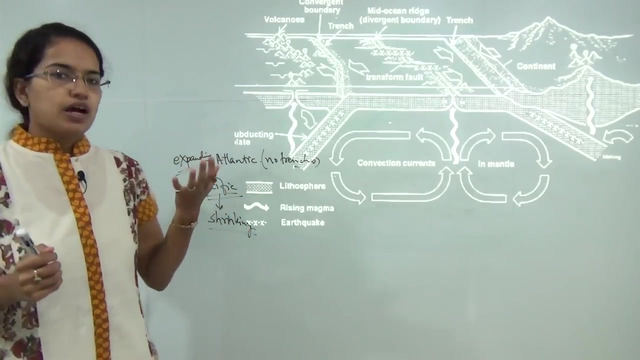 continents drift apart. so, he said, atlantic is expanding. on the other hand, pacific ocean has huge number of trenches. as a result, pacific ocean is shrinking. so these were the two findings that he tried to uh explain. and he said: if there is no subduction, what would happen? so if there is no subduction, that is going here, it will push the continents apart. so if there is no subduction, it would push the continents apart. so if there is no subduction, it would push the continents at a faster rate. so the north america, so the american continent and the african. 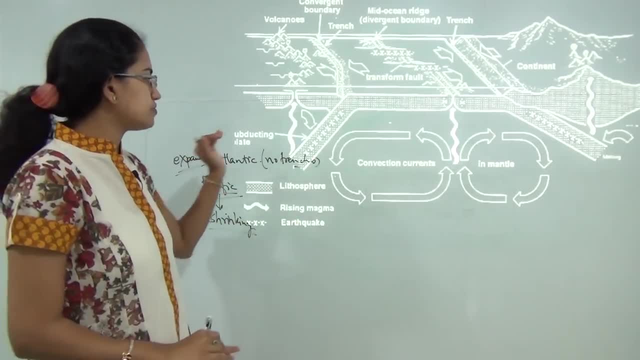 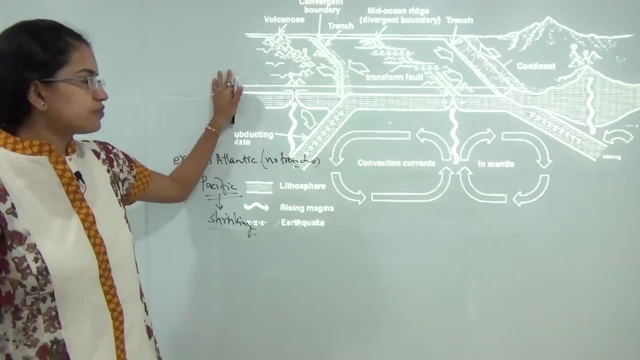 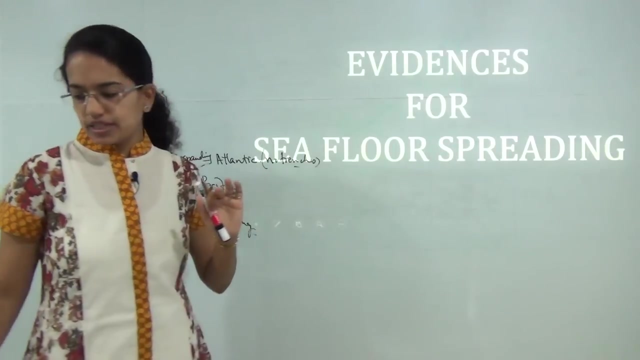 continent are being pushed apart at a higher rate because of this region, because of the lack of subduction zones there. now, the next important concept- so we've talked about the process of sea floor- is spreading and the mechanism of sea floor is spreading. the next important thing is evidences. 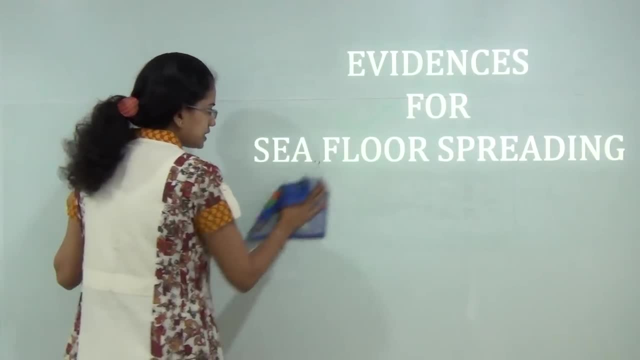 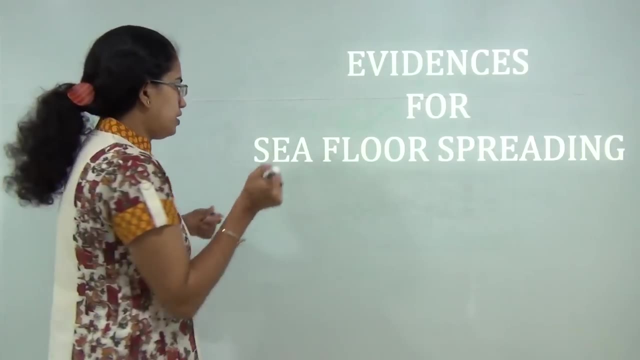 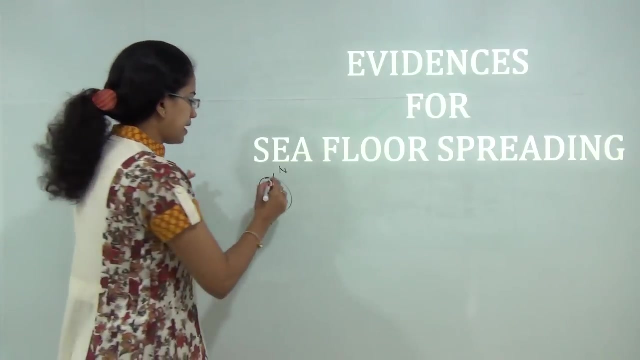 that support the sea floor is spreading. now, when we say the evidences that support the sea floor spreading, the first and the foremost is the magnetic reverses. now, under geomagnetism, we'll study. you have the earth's north pole and the south pole, and then you have the magnetic poles. 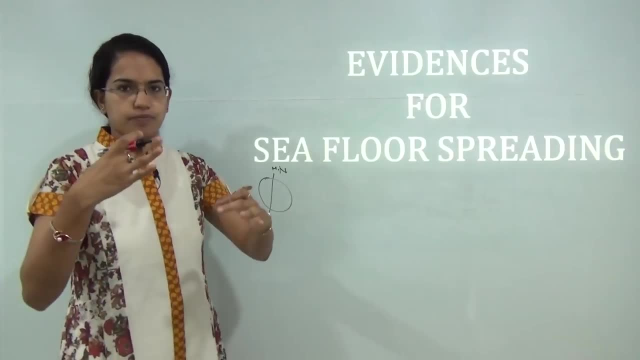 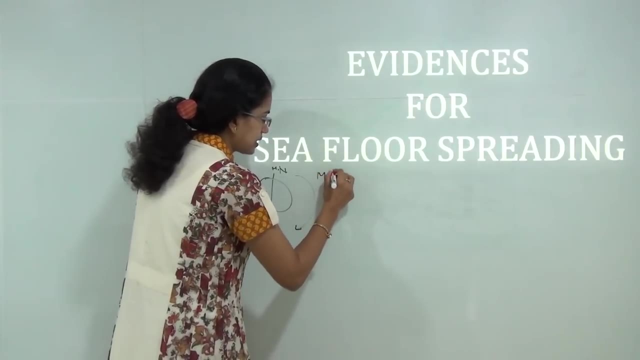 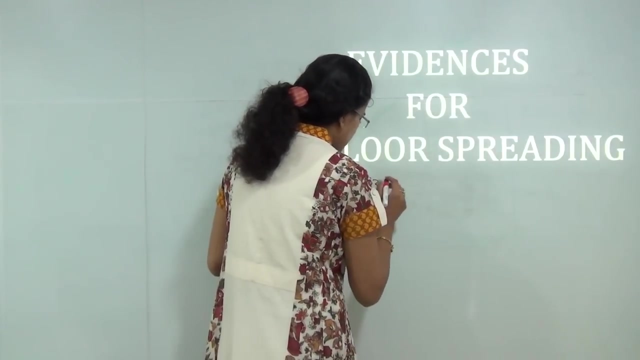 but the magnetic poles keep on switching. when i say keep on switching, that means this becomes the magnetic north, and this becomes the magnetic north and this becomes the magnetic south. and these kinds of switches over the past thousands of year have taken nearly, have taken place nearly 173 times. you have seen such polar reversals and 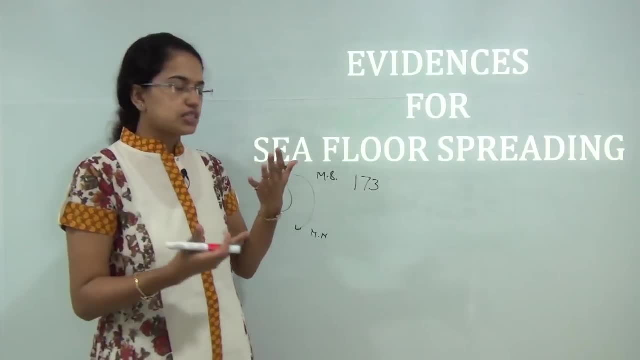 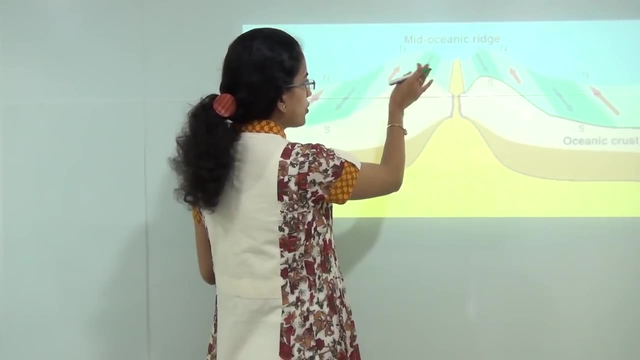 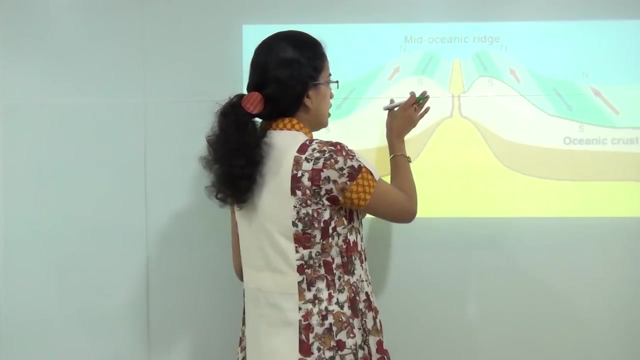 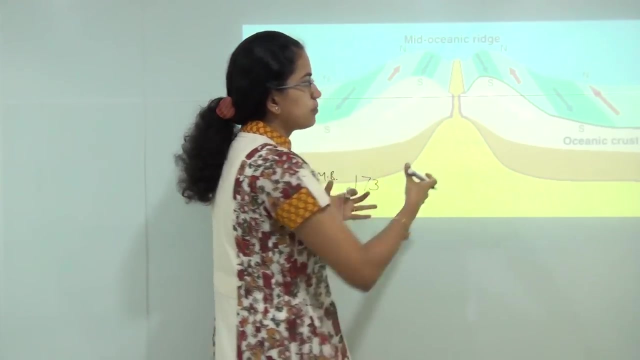 because of these polar reversals, what is happening is you have changes in the polarity. so what can be seen here is you have a series of old rock, new rock, old rock, new rock, and that's due to the switches in the polarity, or the magnetic reversals, that takes place. so, because of that, when henry has tried to study the 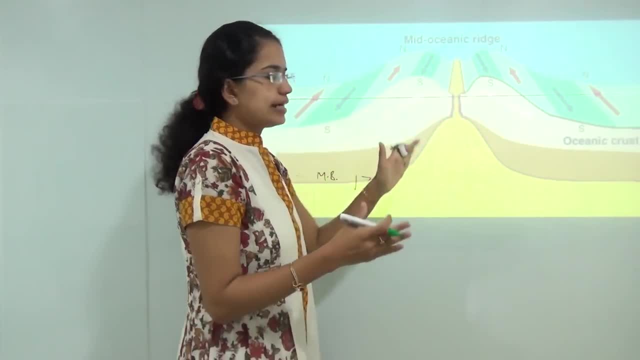 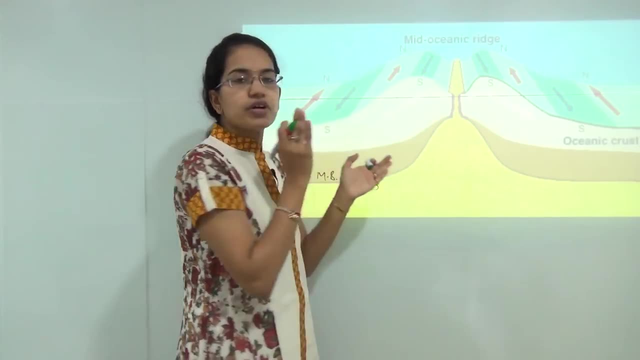 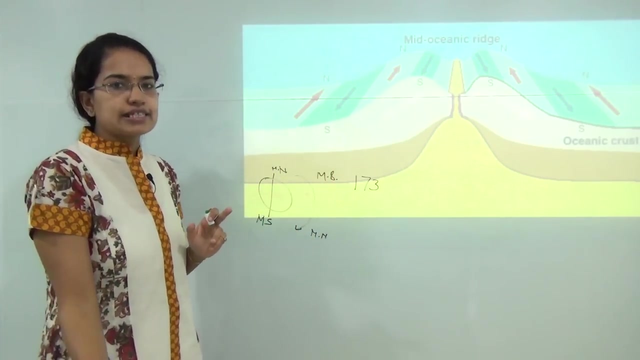 ocean floor. he said there is not a clear evidence that we can find all the new rocks together and old rocks towards one side. rather, there is alternation of a old rock and a new rock. so that was one of the major evidences that confirmed this. the next evidence was that 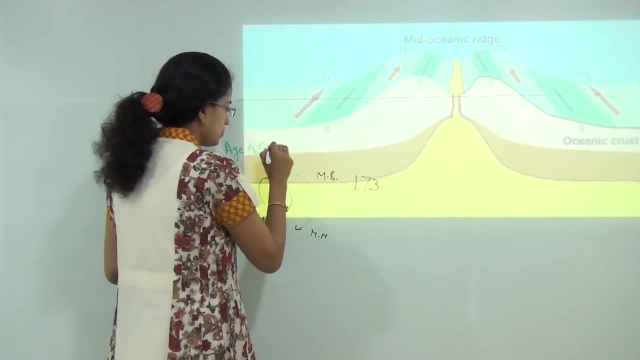 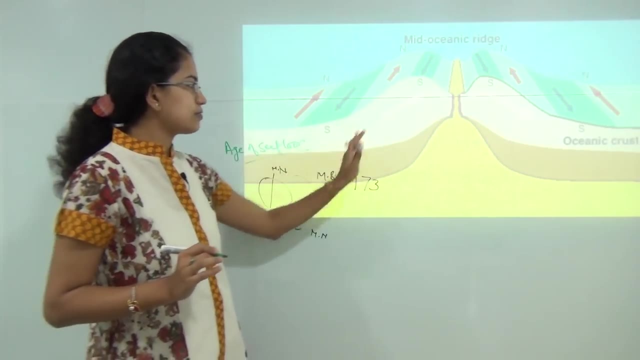 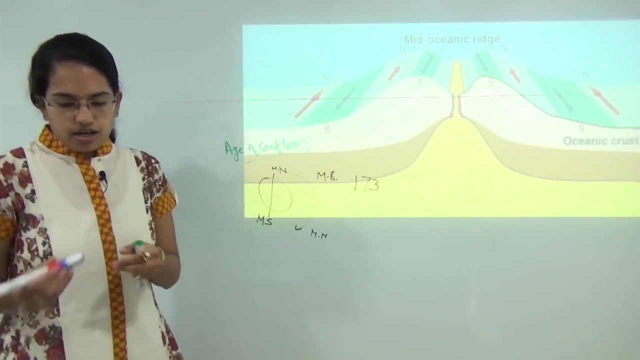 the age of the sea floor and that was determined, again by the polarity. so you can say, due to the magnetic polarity, these, this region of the sea floor is old, this region is new, this region is old, and so on. then he talked about that if continents would be one, 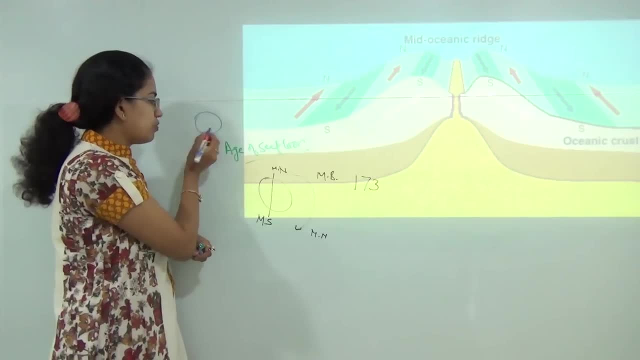 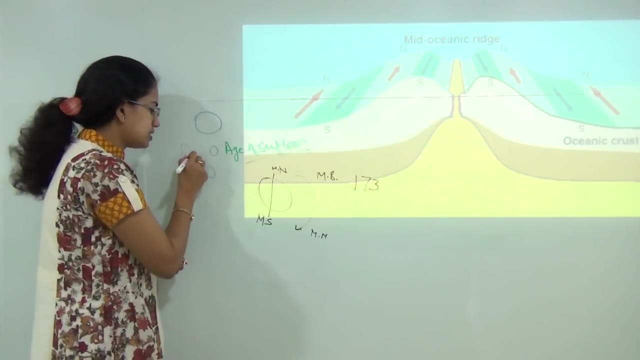 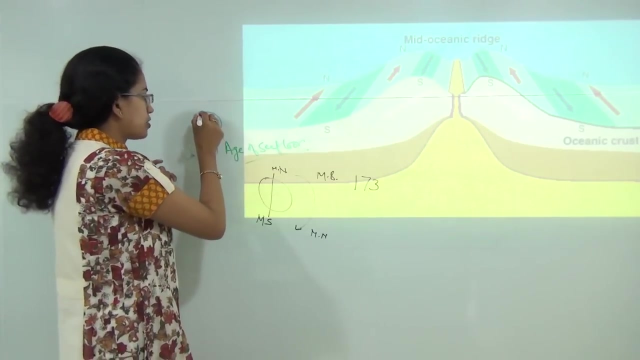 what wegener suggests, then sea floor is spreading. how would we understand that? so he said, there were already, continents were apart and sea floor is spreading. just help them to drift further apart. so rather than considering the assumption of wegener that continent is one single mass, he said: